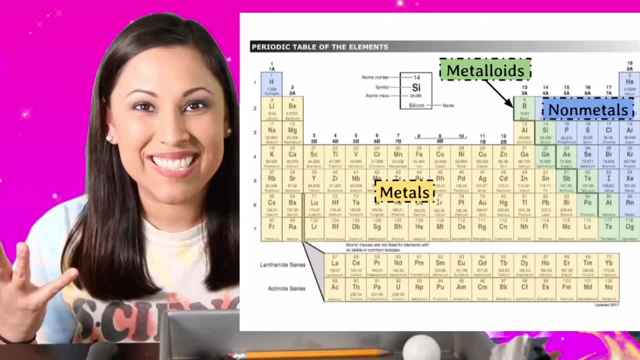 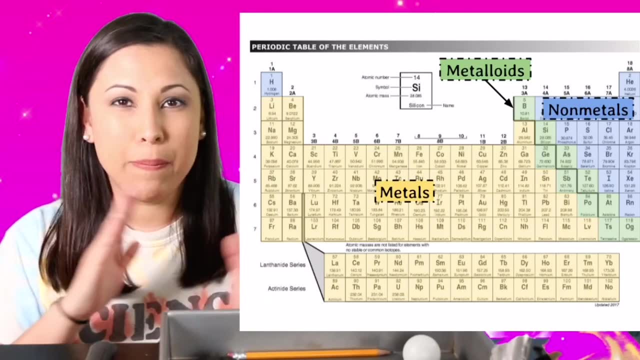 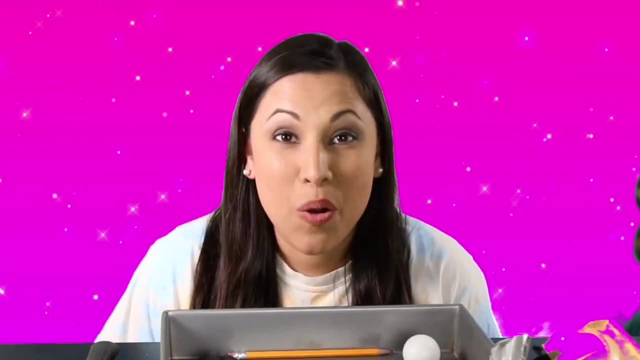 carbon helium. yes, and then in the middle you'll see the metalloids. So the metalloids are in the middle and we're going to explore a little bit about why- And those are located on the staircase. So I brought a few examples of some of the elements with me today so you could see some of their properties. 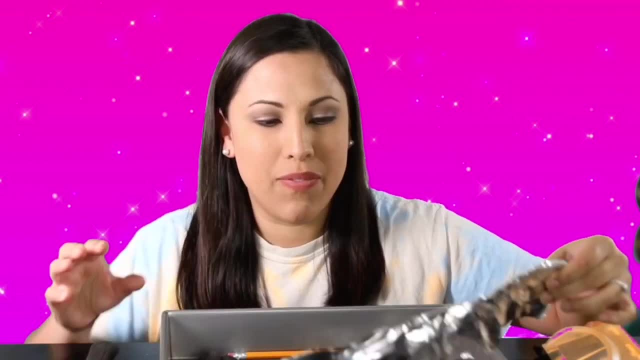 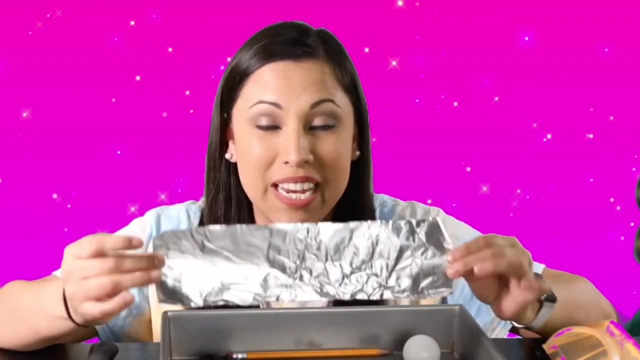 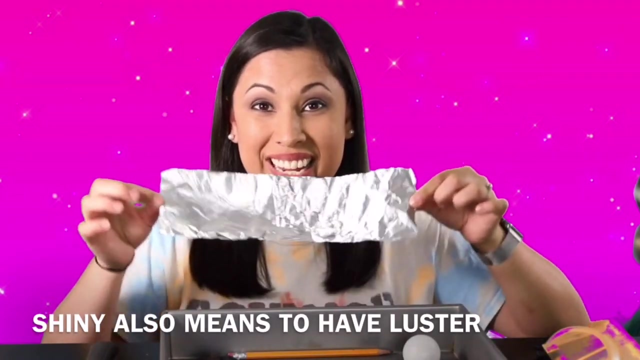 Let's start with one. I know that you've seen before. Yes, this is a piece of foil, Everyday item I know you've seen, probably used. And what are some properties about this? It's shiny. It can change shapes, right. 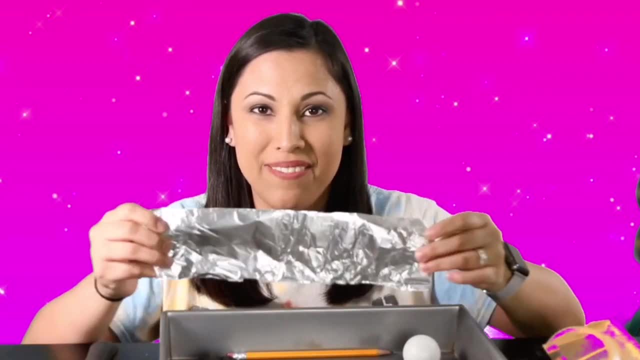 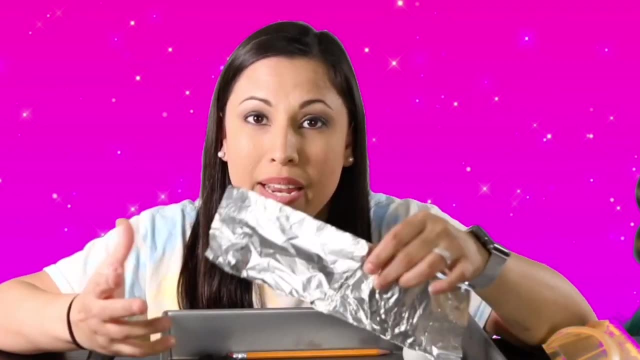 We can wrap it around whatever kind of container we have And it's pretty durable and we can't really break it. We can tear it because it's a thin sheet, But the great thing about metals is that they are malleable. Can you say that with me? 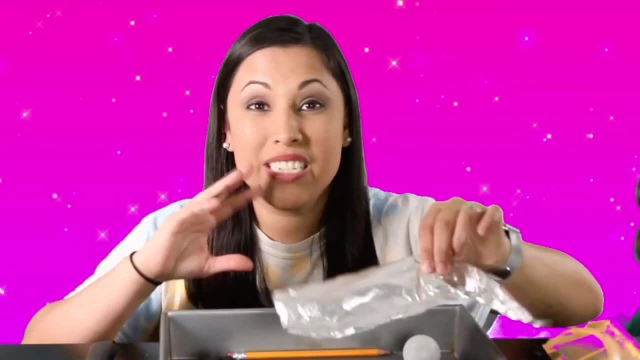 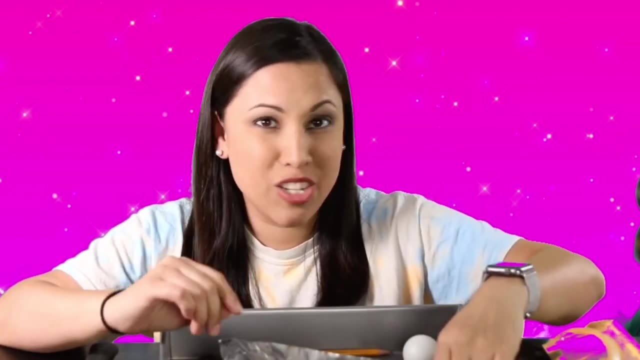 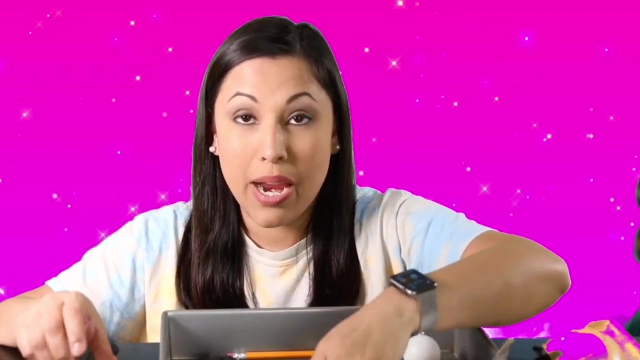 Malleable. So that just means that we can change their shapes and they wouldn't break. So, like metal, we can make it into sheets, We can make it into wire or something else you've seen before- Coins or change. So if I took a hammer and try to hammer these pieces of this quarter and this penny, 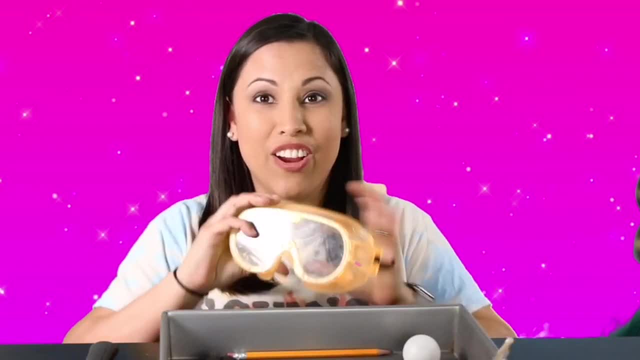 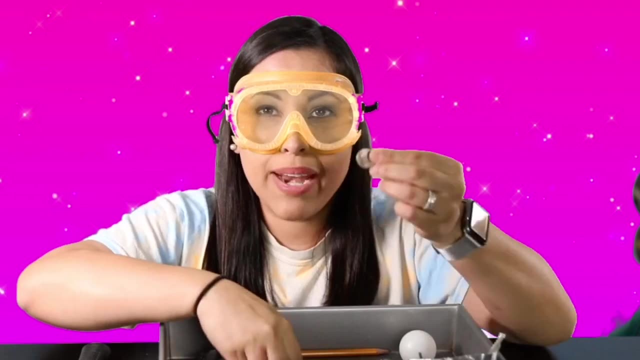 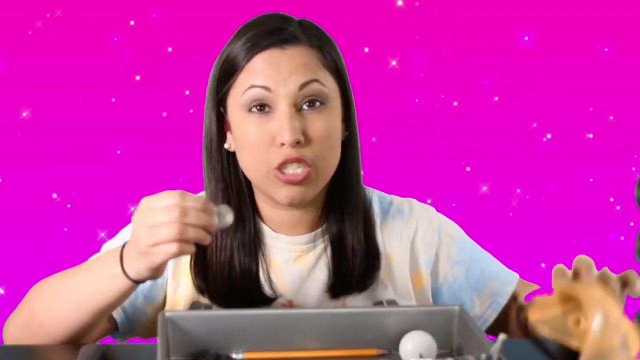 it probably wouldn't break. Let's try Safety first. Not at all. So they might have dented a bit, but they're not going to change shape or they're not going to break, So they're malleable and they're also pretty strong. 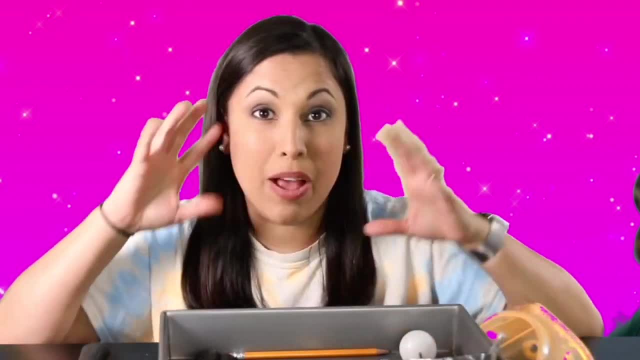 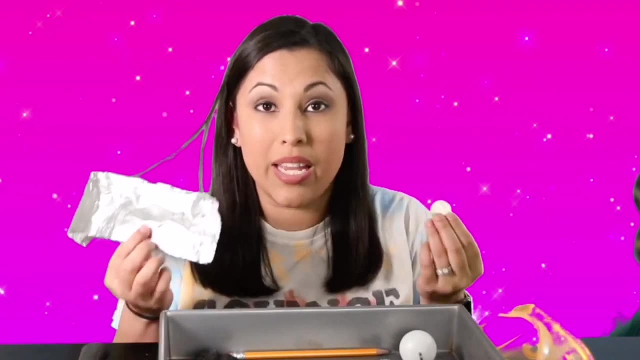 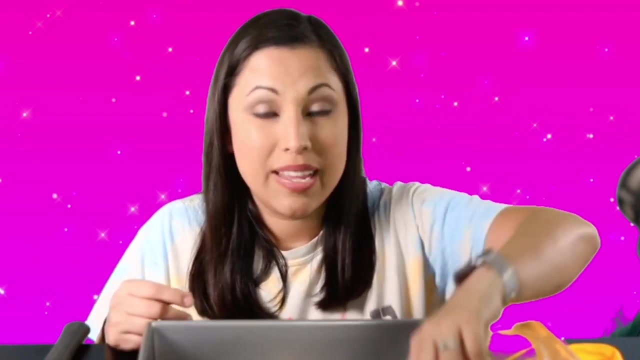 So we also call that ductile. Think about duct tape. how strong duct tape is. So those are metals And also, if you notice, metals are usually solid at room temperature. Okay, another property of metals is what we call conductors. 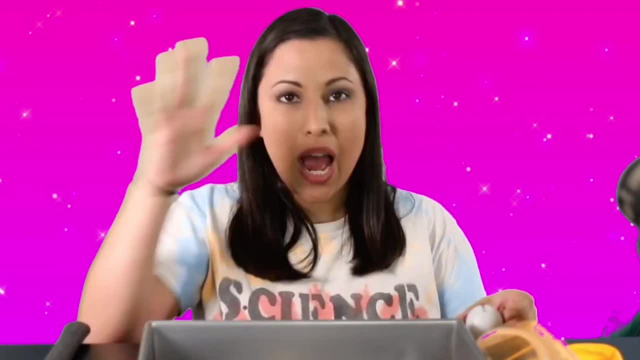 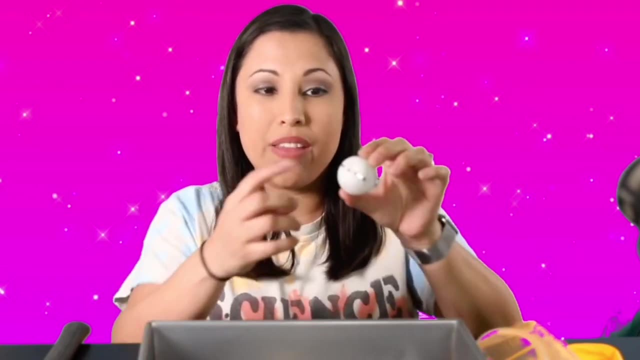 That means that they can conduct electricity. They can conduct electricity or allow electricity to flow through. So I brought with me an energy ball. This is like a little mini circuit, And if you connect these two metal pieces then the circuit will be complete and something will happen. 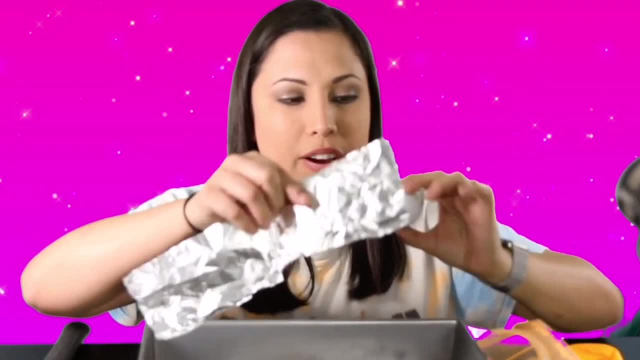 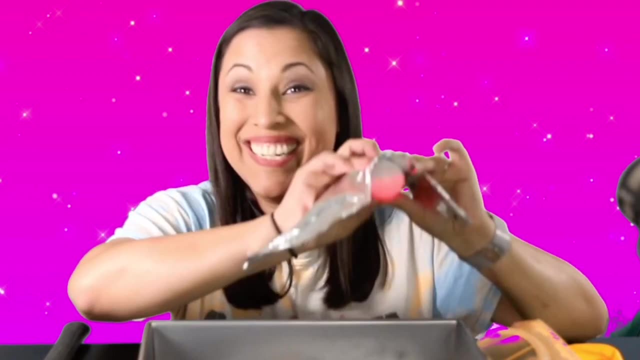 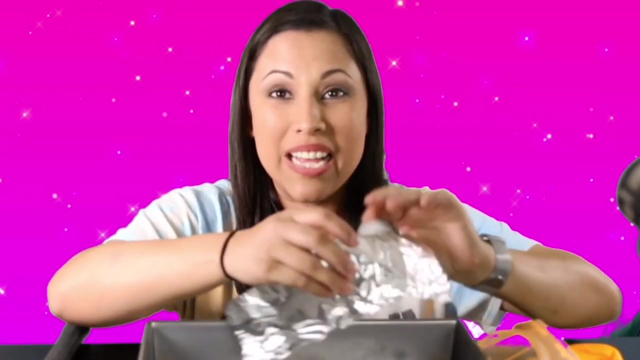 So let's see, We're going to try our foil first and I'm just going to connect one side to the other. So it's lighting up and it's making the noise. So that's what we call a good conductor. If we also use our coins, our other metal, 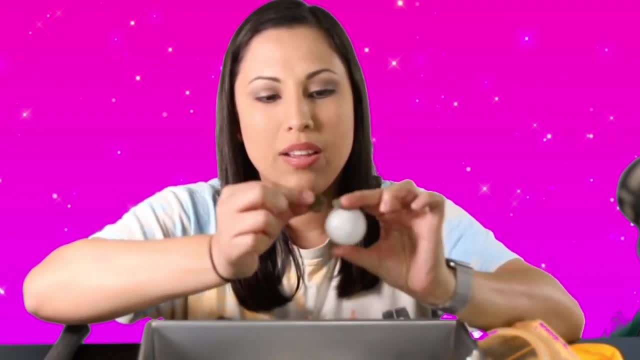 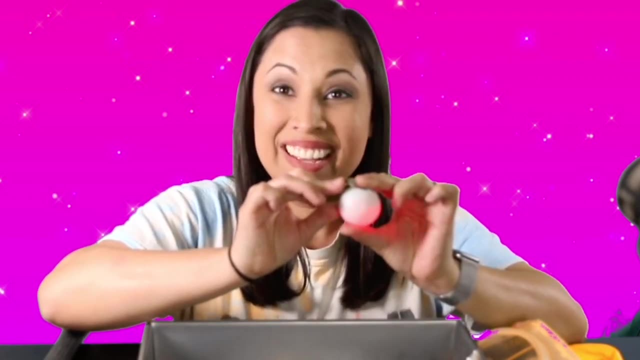 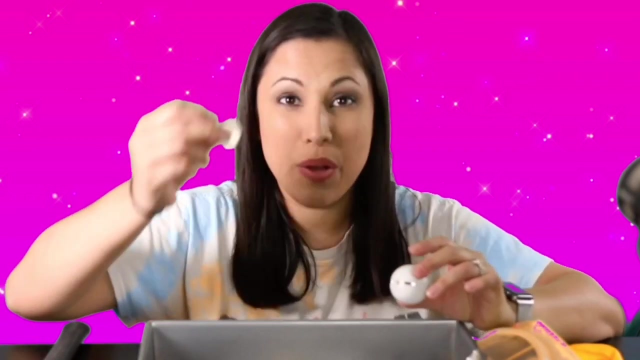 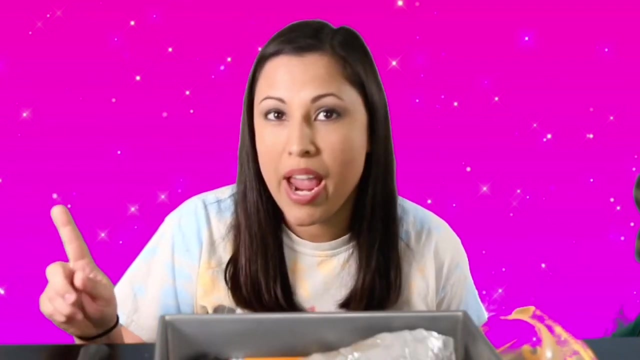 we can also test it out. Doesn't quite reach, so I'm going to use both. So they both conduct electricity well also. So metals are good conductors. They do allow electricity to flow through. Okay, next We're going to skip over to the other side of the periodic table and talk about nonmetals. 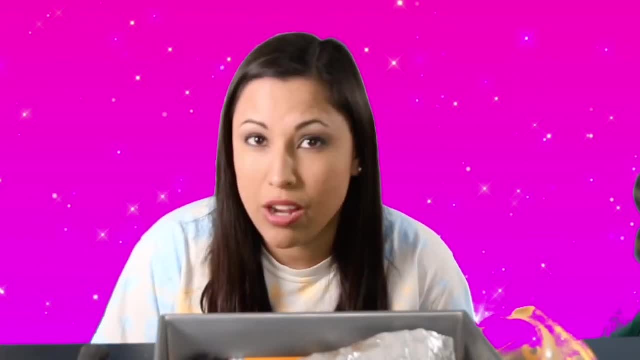 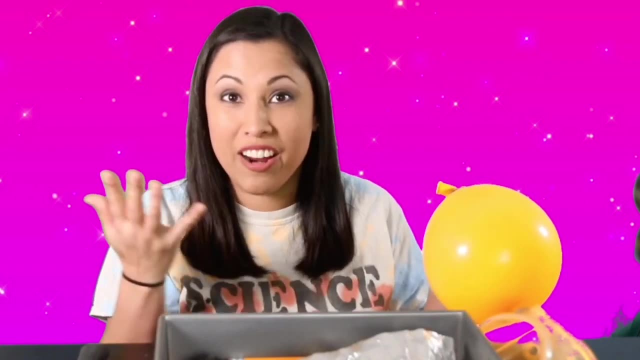 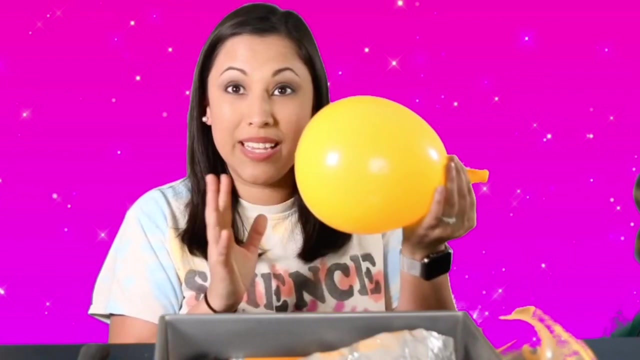 So what are some nonmetals that you recall seeing on the periodic table Right? most are gases. So whenever you think about nonmetals, you probably think about gases at room temperature, Just like this gas that I use to blow up this balloon, or gases like helium. 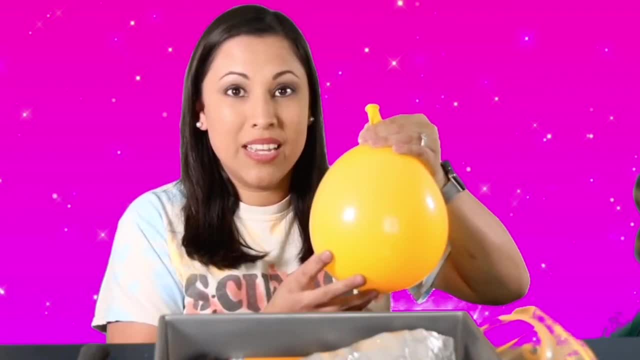 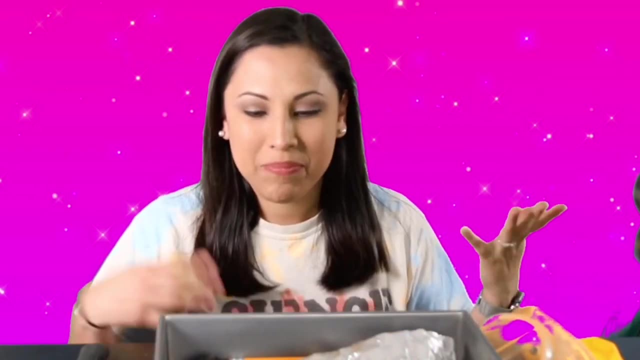 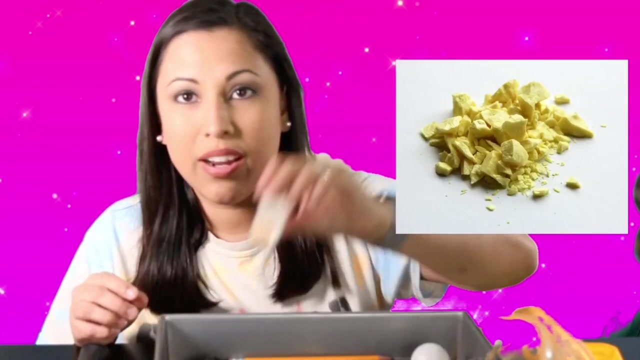 we use to also blow up balloons, But all the air around us, So nonmetals are usually gas at room temperature. All right, I do have another example of a nonmetal, So here I have sulfur. So sulfur, as you can see, is dull. 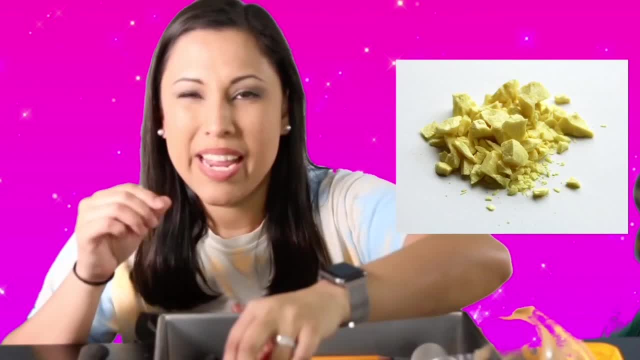 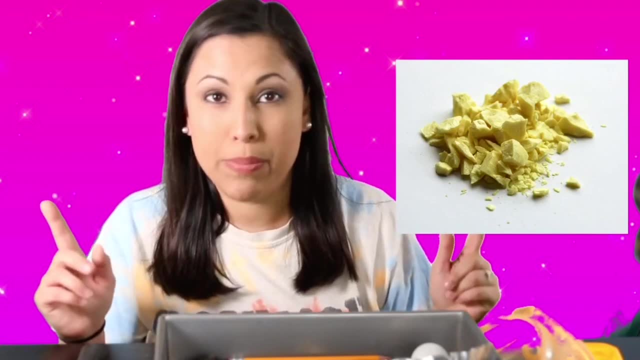 So you can also probably see in the picture a little bit better. It's kind of like a powder, like or can be, because it's so brittle or breaks easily. Can you say that word brittle with me Brittle? So that just means that it breaks easily. 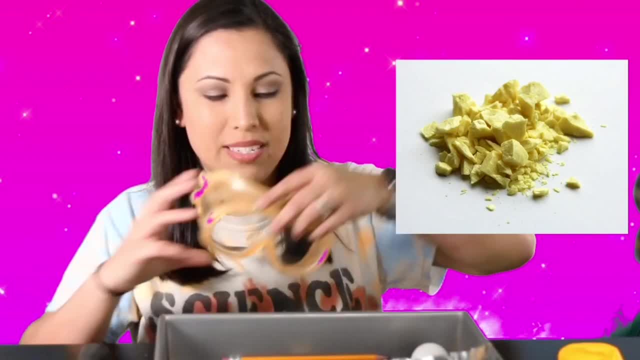 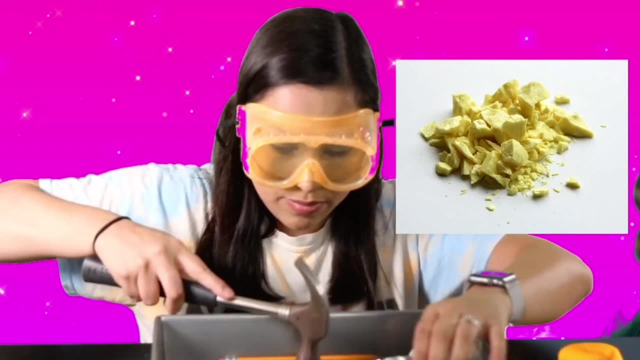 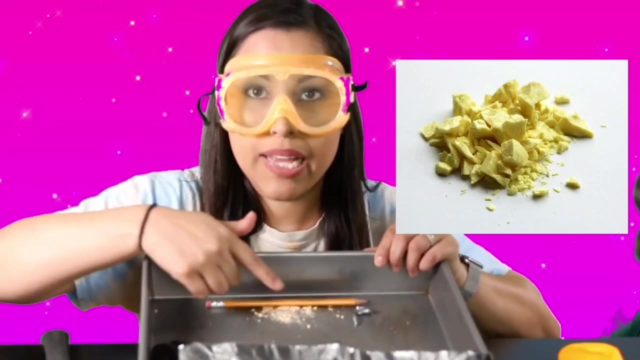 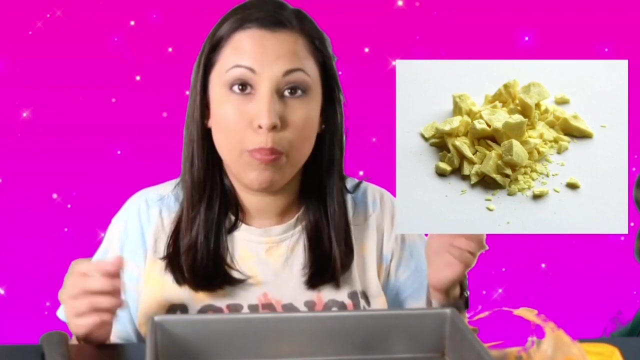 So I have a little bit right here and we can see safety first. If I use a hammer, again what's going to happen. So you can probably see here that it basically turned to a powdery substance. That's because nonmetals are brittle or break easily. 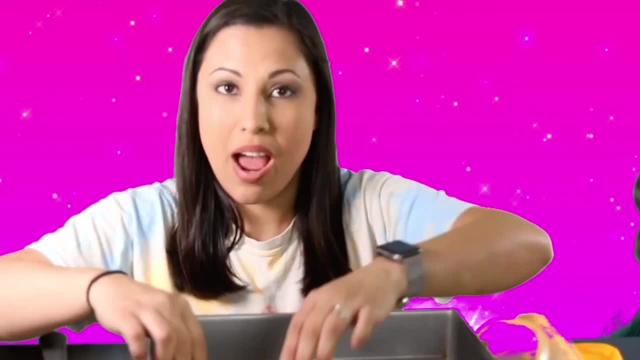 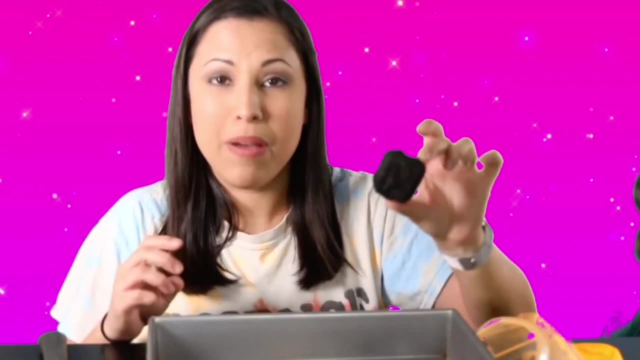 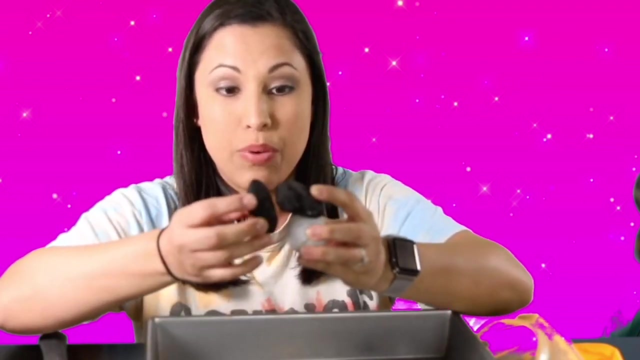 I also brought with me another piece of nonmetal that I know you've seen before. Yep, you guessed it: charcoal. Charcoal is made up of mostly carbon. So if I use my energy ball again and I test out charcoal, let's see what happens. 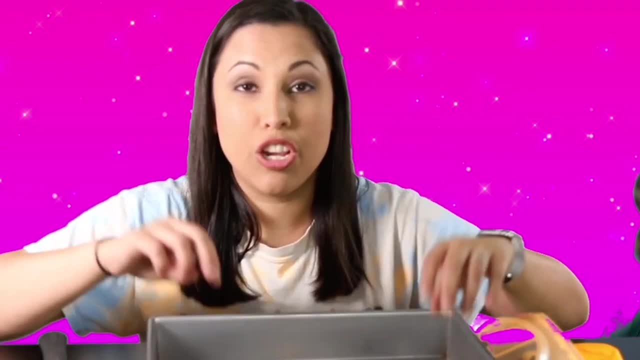 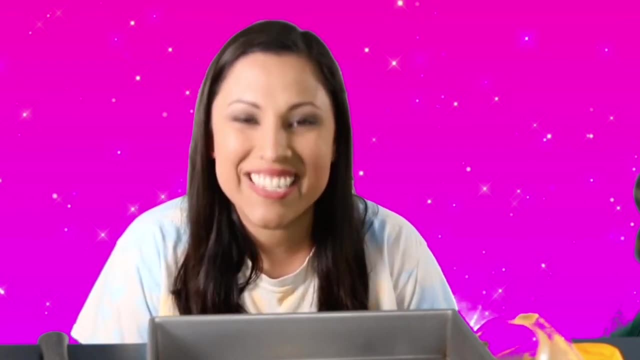 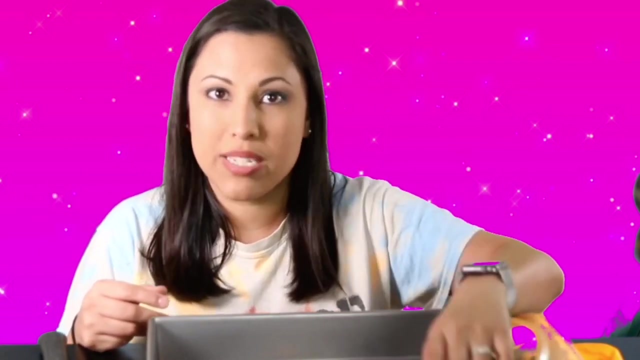 Nothing That's because nonmetals are good insulators or poor conductors. Can you say that word insulators with me? Insulators, Good job. That just means that they do not allow electricity to flow through. Hence why our energy ball didn't work. 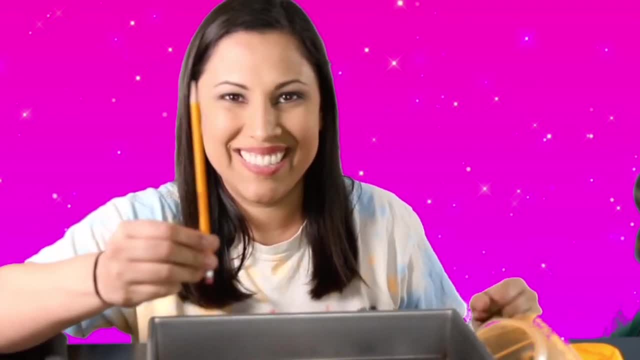 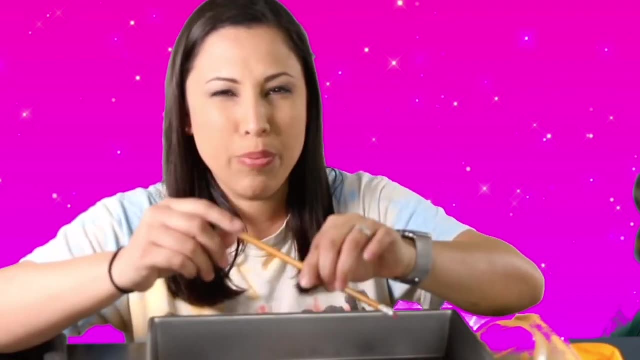 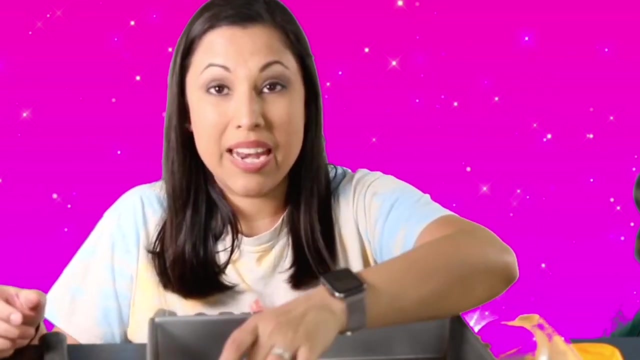 So I brought something else with me that you probably will recognize. Yes, So graphite, or the lead of pencils, is also made up of carbon. So you probably noticed whenever you have a piece of lead it breaks easily. It's brittle. And now if we try our carbon with our charcoal? 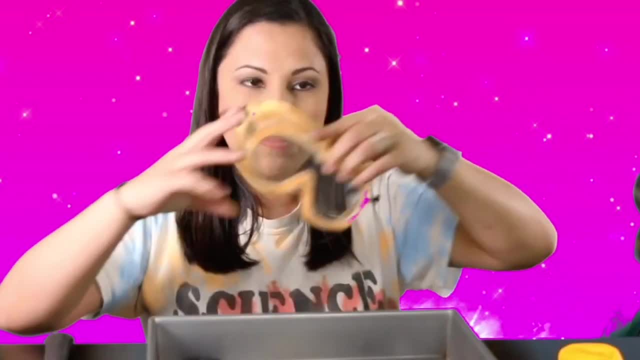 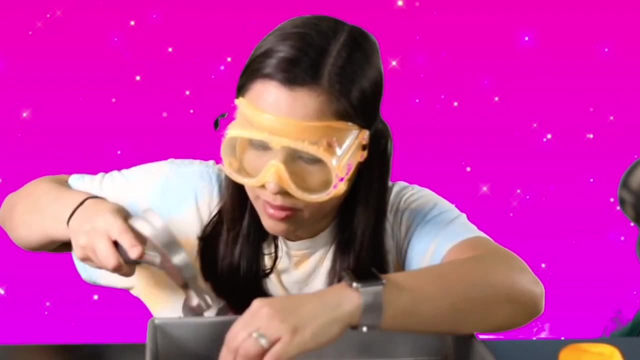 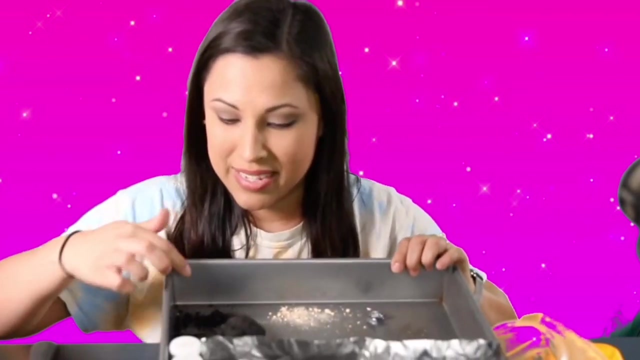 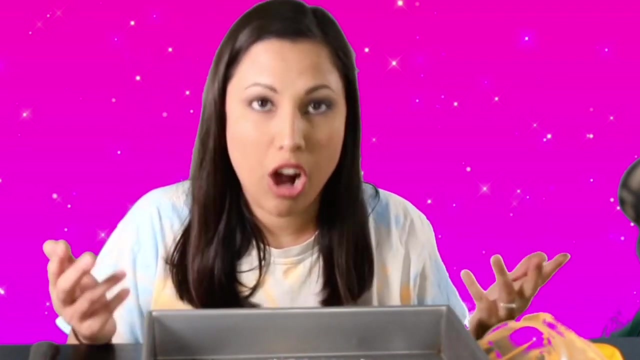 try to break that with our hammer. Let's see Safety first. All right, That was a little bit tougher than our sulfur, But, as you can see, it did break down and some of it did turn into a chalky substance. So charcoal or carbon is also brittle. 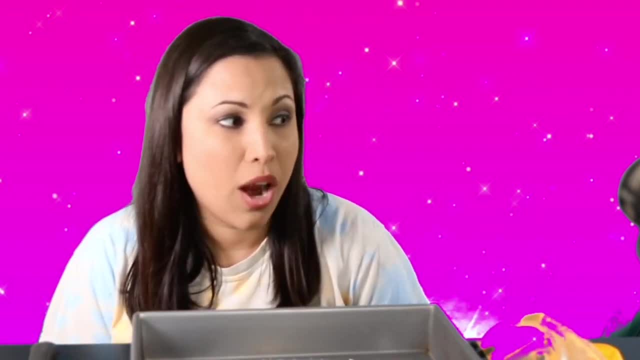 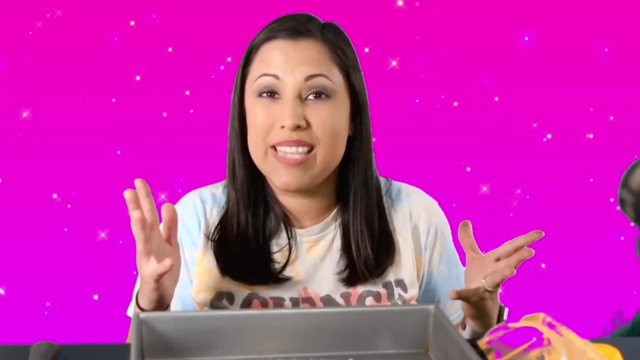 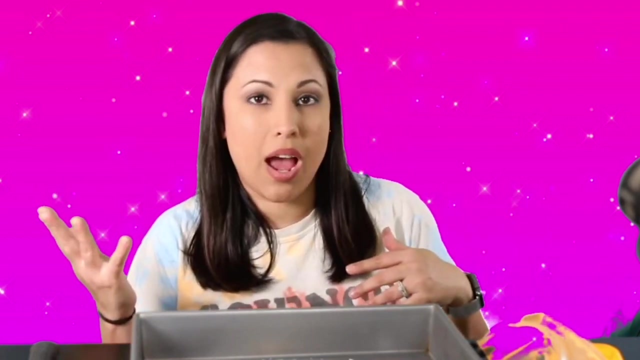 Okay, Now let's talk about our metalloids. So our metalloids are in the middle in between our metals and our nonmetals, And that's because they take some of the properties of both. So, depending on the element, they can act more like a metal or more like a nonmetal. 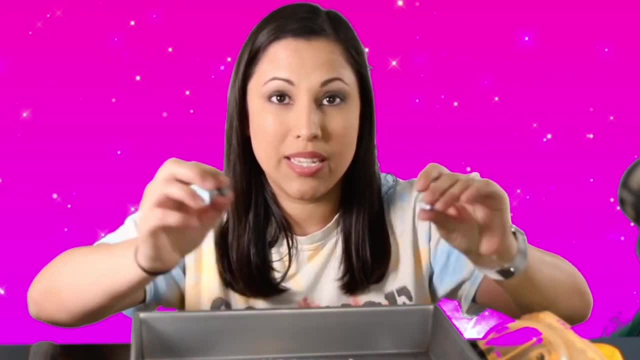 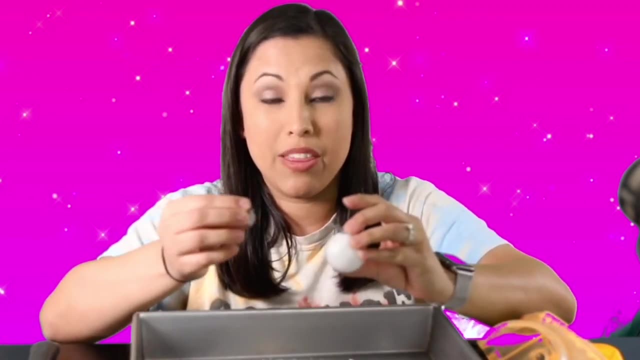 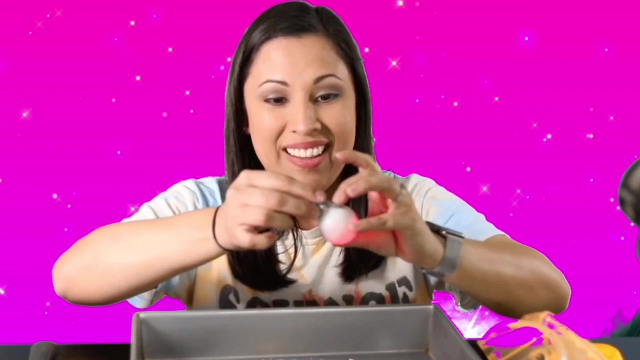 But I think one of the biggest things that you'll notice is that they are semiconductors. Let's see, What does that mean? Are they going to conduct electricity? Yes, they do. So our metalloids are semiconductors. 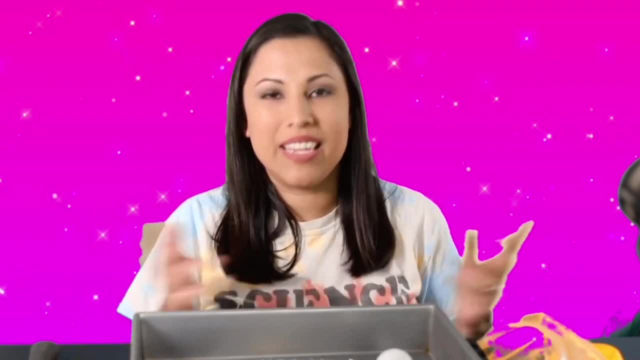 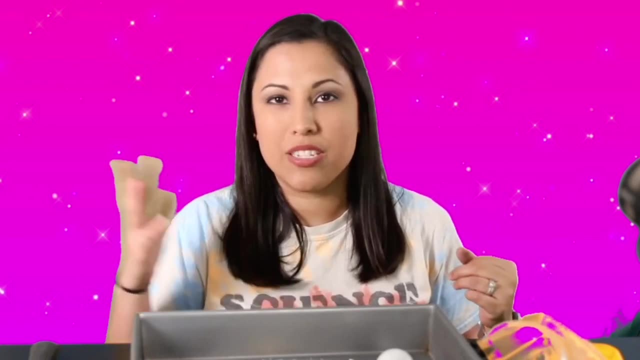 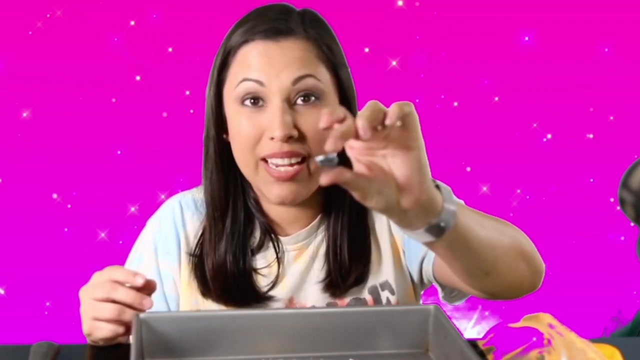 Can you say that with me? Semiconductors, Exactly So, they do conduct electricity, They're just not as great conductors as metals and they're not insulators like nonmetals. But you can see, our silicon is shiny like a metal. 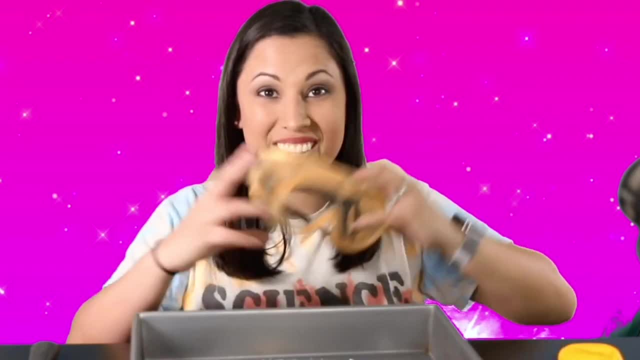 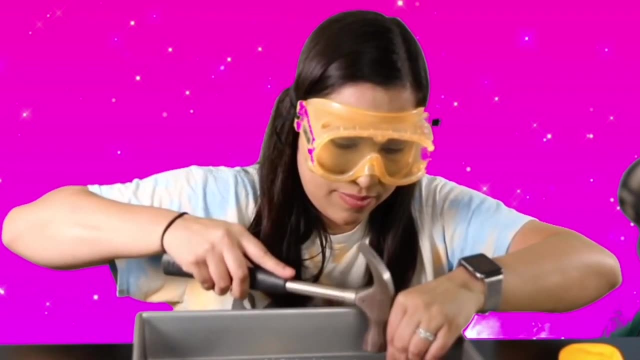 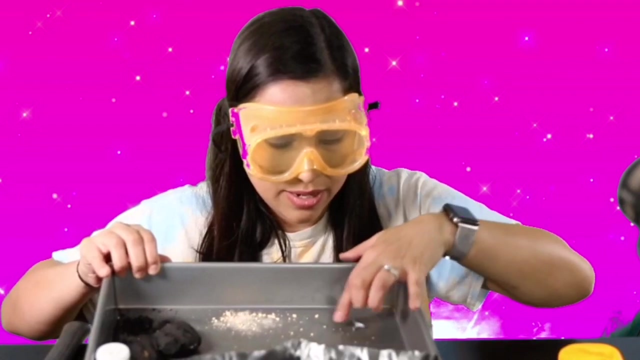 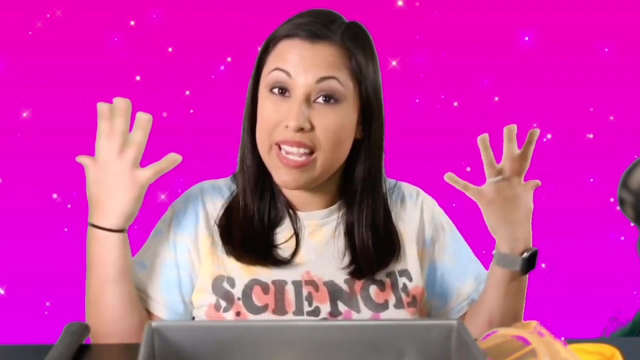 Let's see if it's as brittle- Safety first. So you can probably see this here. It did break pretty easily, So it is brittle, So it has properties again of both metals and nonmetals. That's why they're in the middle that staircase. 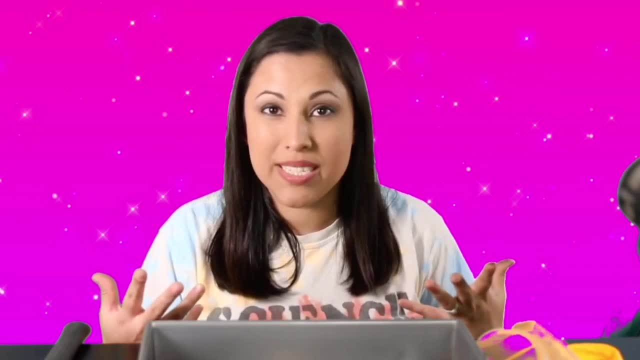 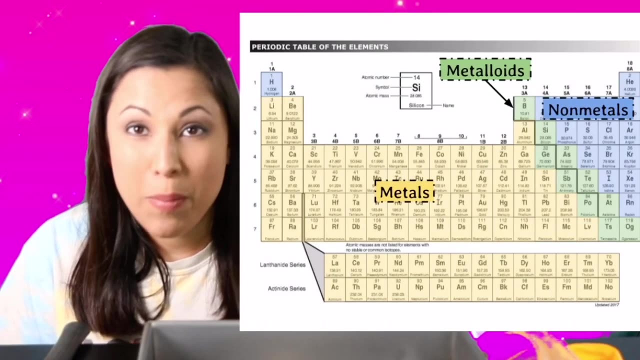 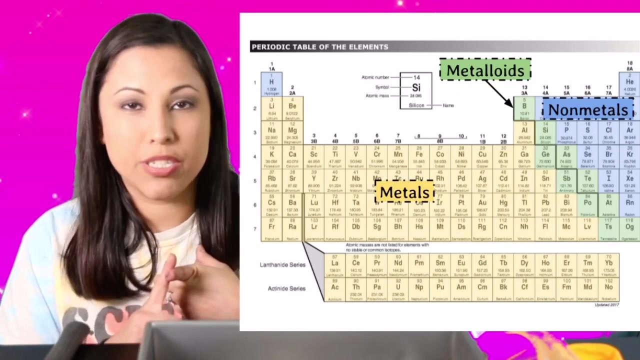 because they're kind of in between, They are called metalloids. So the main property of metalloids are being semiconductors. So remember our metals take up most of the periodic table and that's on the left side. Remember they are solid at room temperature. 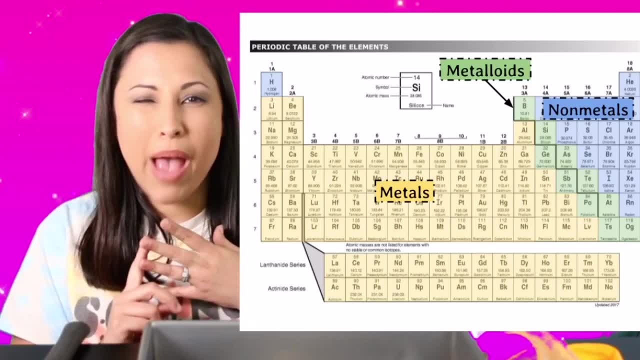 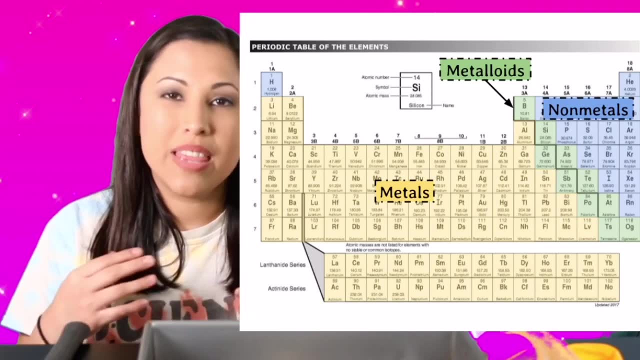 They are great or good conductors, They are malleable and ductile. We can change their shape. So if we take a look on the other side of the periodic table, the nonmetals, then we know that they are mostly gas at room temperature. 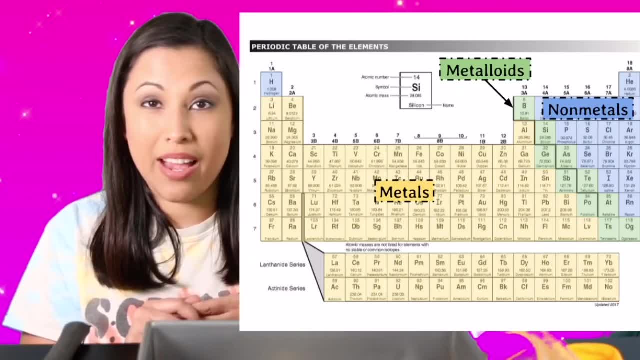 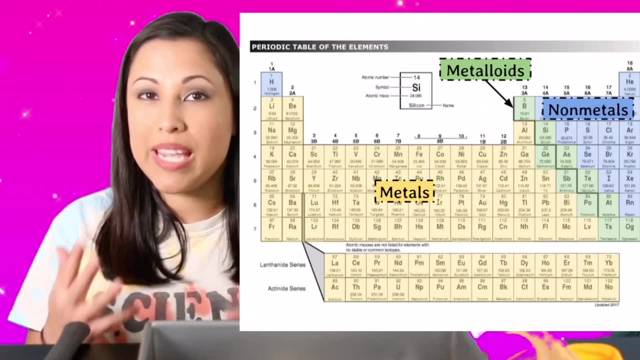 but they can be solid. They're going to be dull, not shiny like our metals, and they're poor conductors, or what we call insulators. They're also brittle, which means they break easily, as we saw with our sulfur. So then we look in the middle, the zigzag, or the staircase. 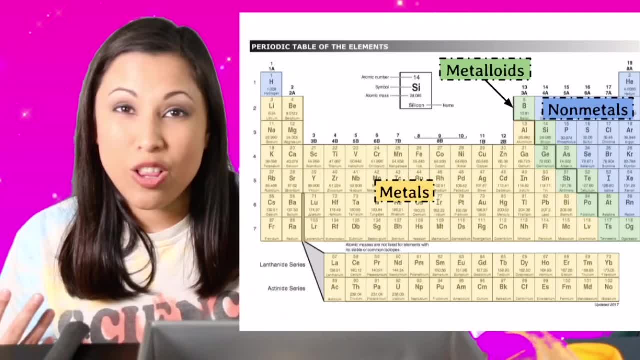 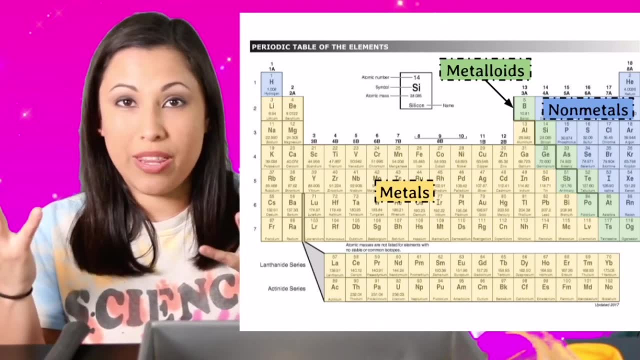 as I like to call it. Then you'll find your metalloids. Remember, they are in between because they act similar to metals and nonmetals, depending on the element. As we saw with silicon: it was shiny but it was brittle and, most of all, 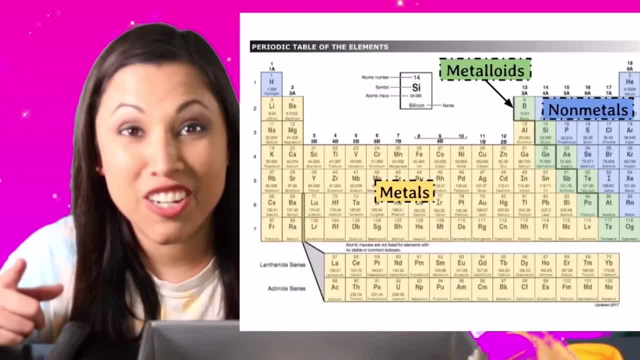 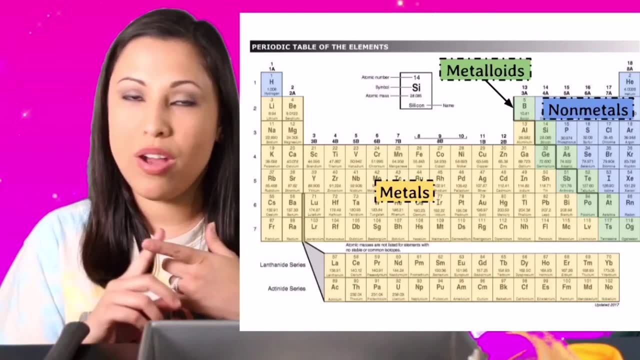 they are semiconductors. So now it's your turn. Find a couple of items you have lying around and try to classify them using the properties we went over today, as either a metal, nonmetal or metalloid, If you're not sure what something is made of. 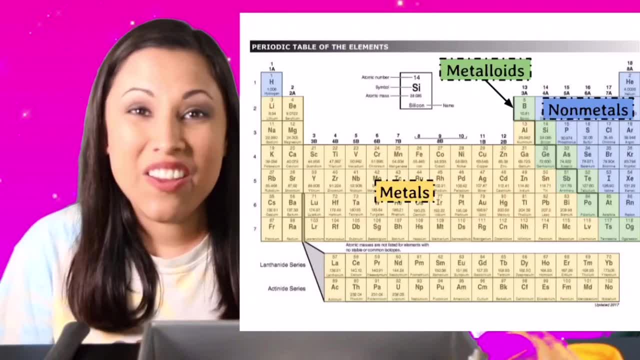 do a little research and try to find out. Thank you for watching and we'll see you next time.